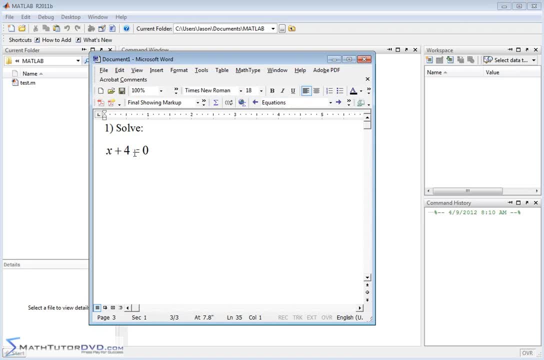 the easiest way to do that is to realize what we have is something on the left is equal to zero. So really we're asking essentially for the roots of this equation. We're trying to find out when this equation crosses the x axis. that's going to be when this guy is. 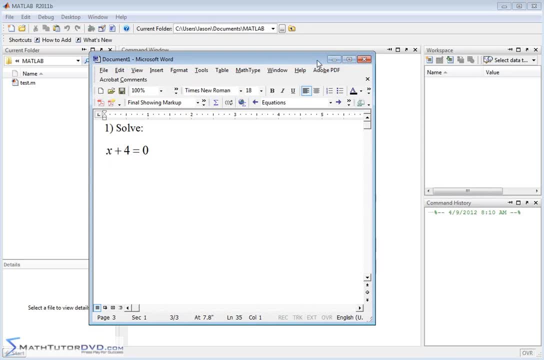 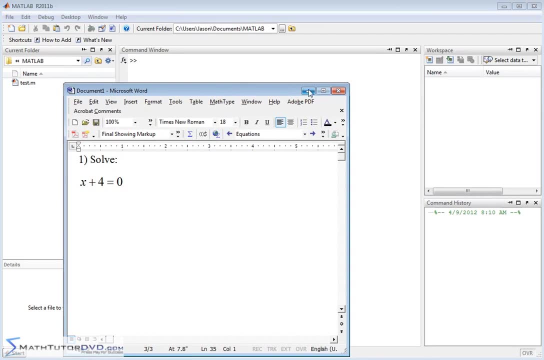 equal to zero. So MATLAB has a roots equation, I'm sorry, a roots command built in and what we need to do is basically solve it. So basically find the roots of this guy here. So this is x plus four, Now what you want. 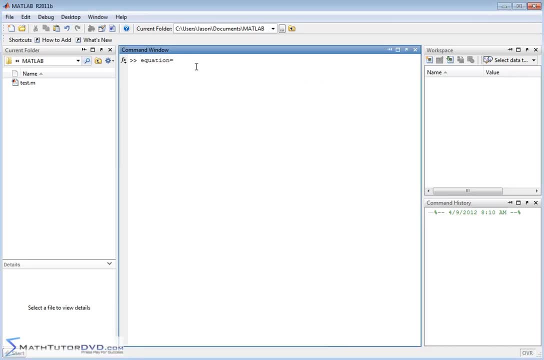 to do is you want to set up an equation and you want to tell MATLAB what the equation is. Now you don't type in the actual equation, like x plus four is equal to zero. You just need to define the left hand side in terms of coefficients. So if I wanted to represent 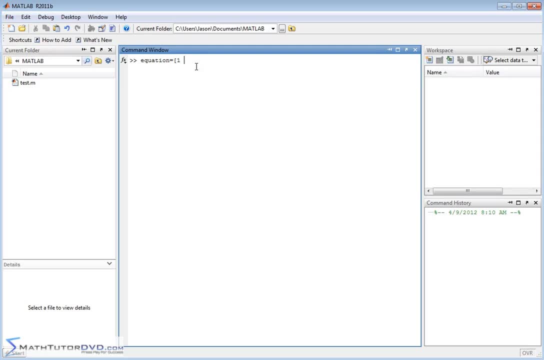 that as a coefficient it would be: one x plus four is equal to zero. So these coefficients really are the only thing that's needed to solve this equation. So if I wanted to do something like this, I'm going to go ahead and do this. So I'm going to go ahead and. 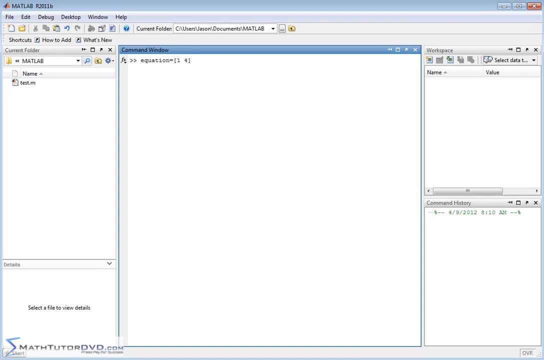 two plus all, x plus four is equal to zero. So this is the right way. So I'm going to then convert this equation into a new Gradient. So remember we're not doing symbolic math right now. We're still using the numeric capabilities of MATLAB. So really, all you're. 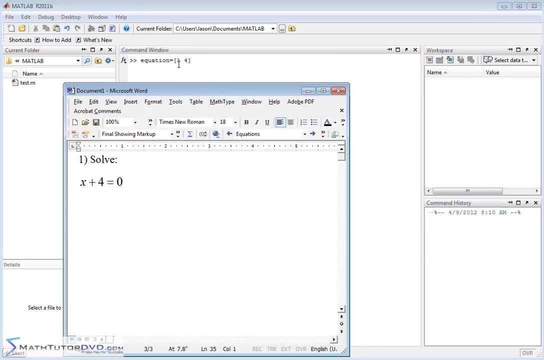 going to do is represent this equation by its coefficients on the left hand side. So one x- that's why we have the one here- plus four- that's why we have the four here. Alright, So these are the coefficients on the left hand side, in descending order. So let me go. 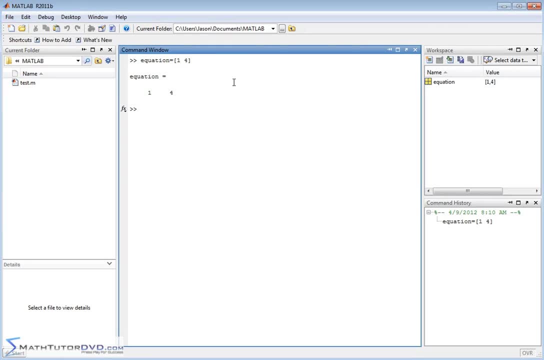 and hit enter, and what's going to happen is we're going to assign this matrix to the word equal". Now then, all we have to do is use MATLAB's root command and pass it the guy that we just defined. So this is an equation. 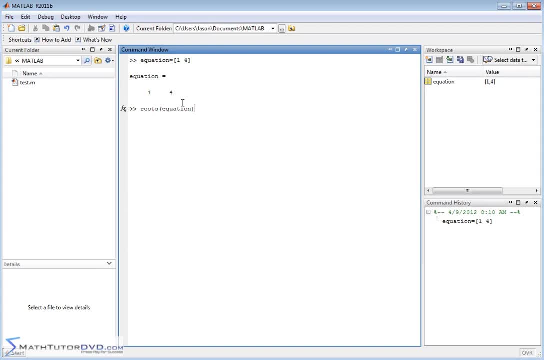 MATLAB knows that when we send something to the roots command, the matrix or the line, the single row matrix that we have is going to be a list of coefficients in descending order. It knows that since there's two coefficients, it has to be 1x plus 4.. 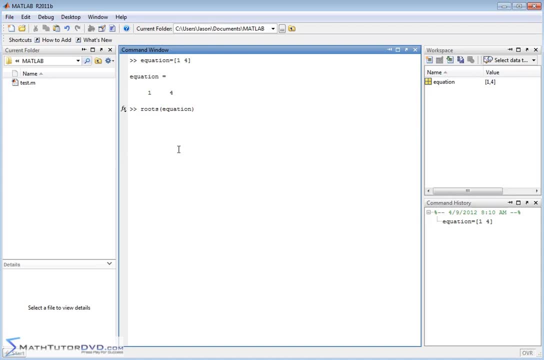 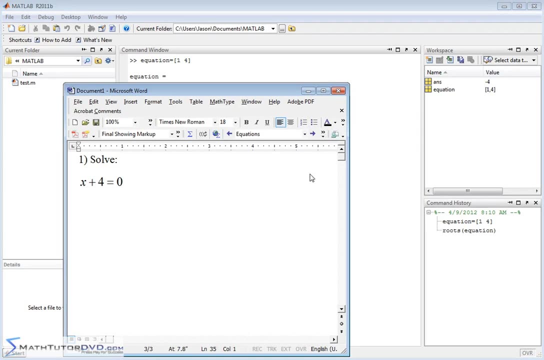 And it knows that it's set equal to zero because we're doing the roots of it, And so then it reports the answer is negative 4, which is exactly what you would expect by moving this over to the other side. So let's get the hang of this with another equation. 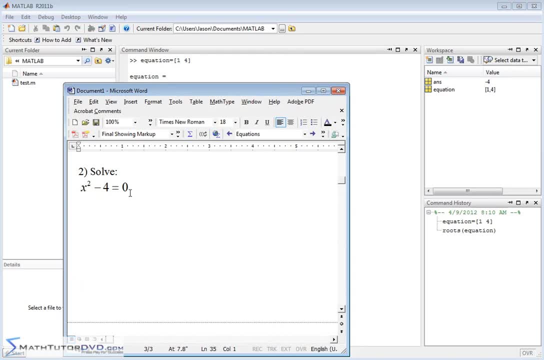 Let's say we have x squared minus 4 is equal to zero. So you can kind of mentally- you know I'm choosing easy equations- you mentally move this over. It's going to be a positive 4. You take the square root. 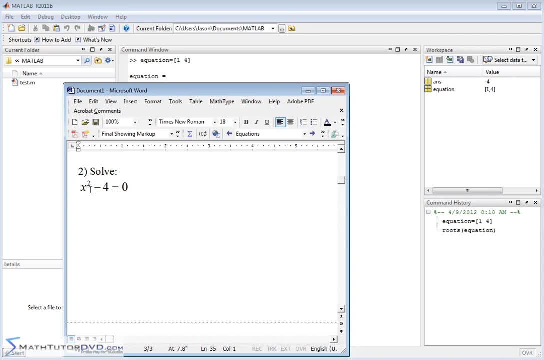 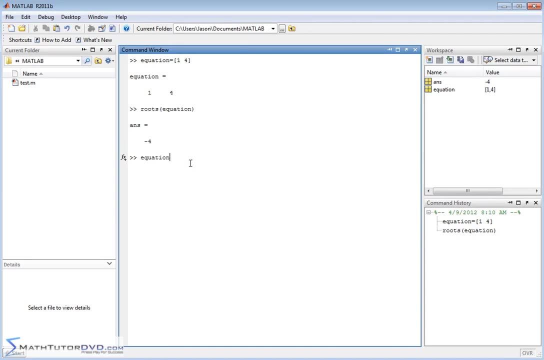 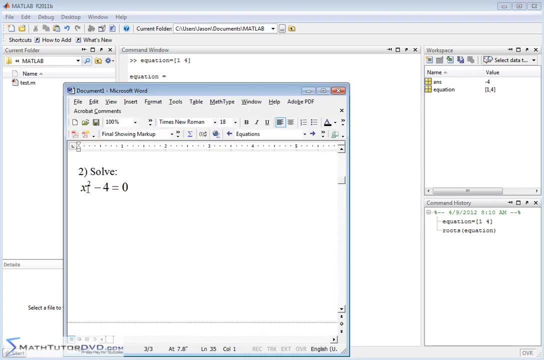 So you should have plus or minus 2 as your answer. So we need to represent this on the left hand side by the coefficient row matrix Again. so let's reassign the variable equation. So what do we have here? It was 1x squared minus 4.. 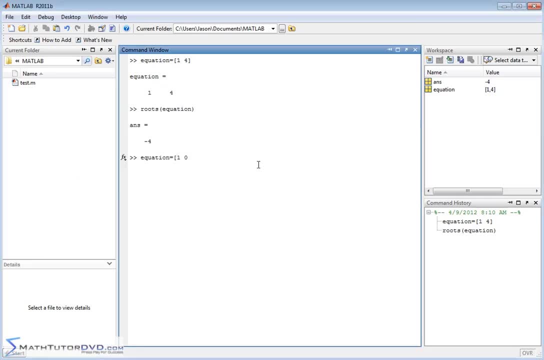 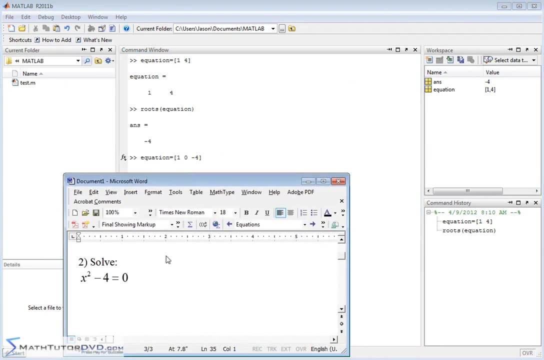 So we have the 1x squared there. plus 0x, minus 4 is equal to zero. Now make sure you understand what I'm, what I'm doing here. What we have here is: when you define this guy here, you need to have a spot for everything. 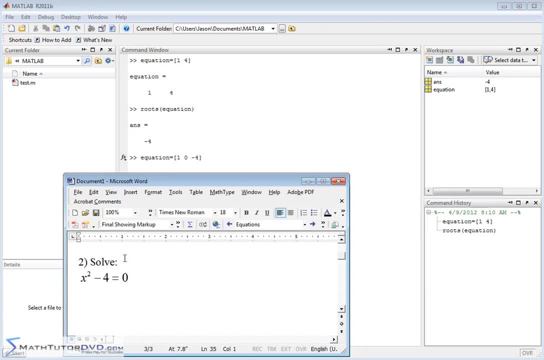 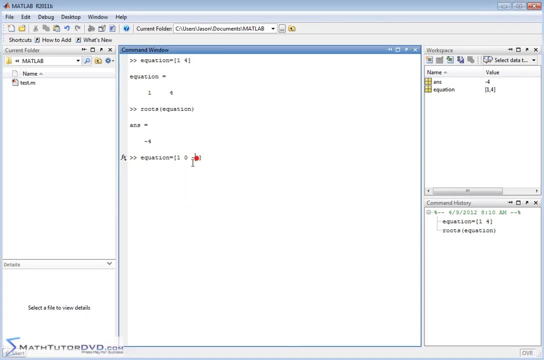 for every descending power of x, So it's 1x squared. There are no x's in this equation, So you have 0x. And then the last thing: the constant on the left hand side is also wrapped up in there as well. 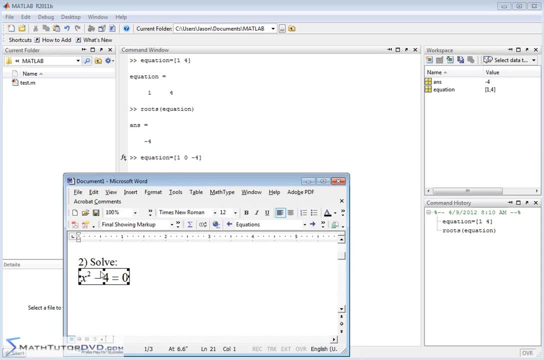 So anytime you have a 0x or anything missing in the descending order of x, you need to make sure and put that in there. This tells MATLAB that this is a basically a second degree polynomial. 1x squared plus 0x minus 4 is equal to zero. 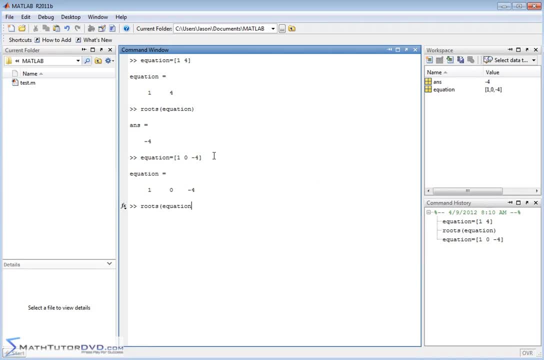 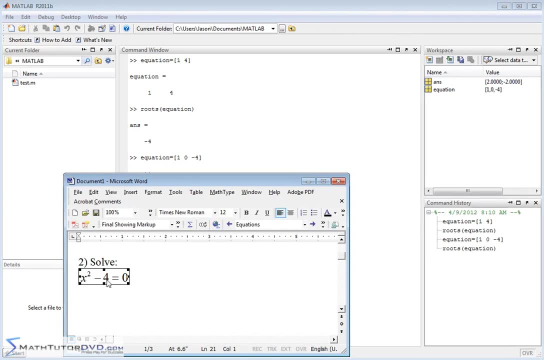 So let's go ahead and set that up and do the roots of equation And it says plus or minus 2, which again is exactly what you would expect. You move this over and make it 4.. Take the square root. You should get plus or minus 2.. 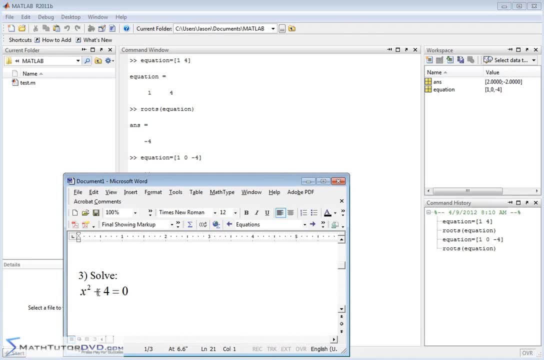 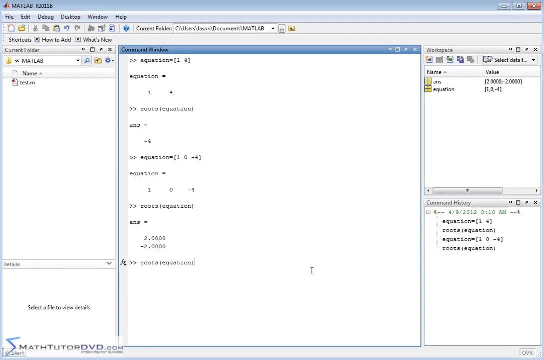 So let's go to the next guy. The only difference between this one and the last one is we change the sign here. Now it's x squared plus 4.. So what I'm going to do is hit the up arrow key and I'm going to retrieve the last command. 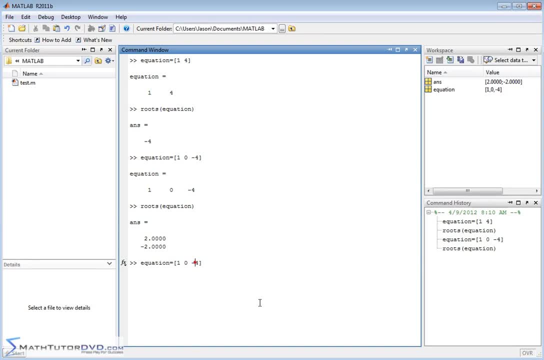 I'm going to do it one more time and retrieve the command before that, just so that I can take this minus sign and basically make it a plus. So that's all. that's different between this problem. So let's go ahead and do that. 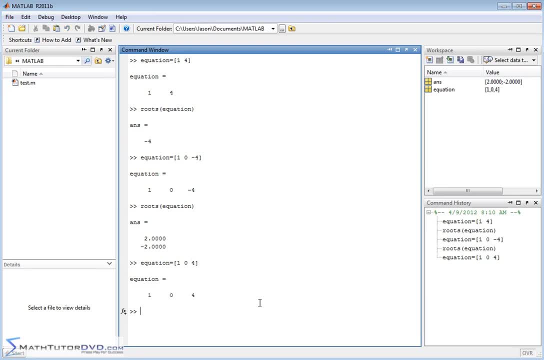 And the last one I'm going to hit enter. So we've defined the equation in MATLAB, or the polynomial we're trying to find the roots of, And then we do the roots of the variable equation that we just defined. Now notice what happens here. 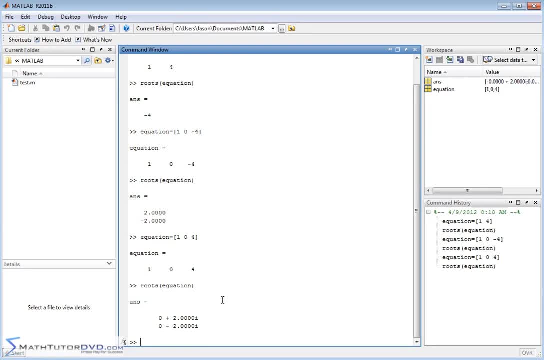 We have a complex answer. So, again, MATLAB has no problem giving you complex answers. Here we have 2i and the other answer is negative 2i, And these are conjugates of one another, which is sort of the rules of algebra. 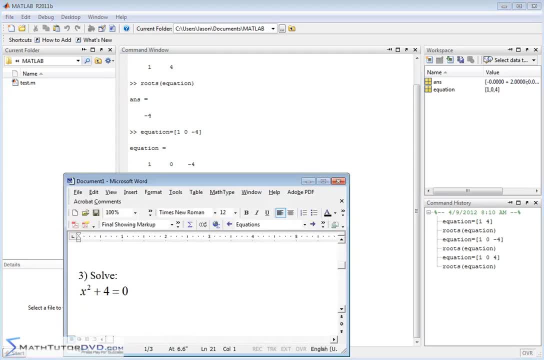 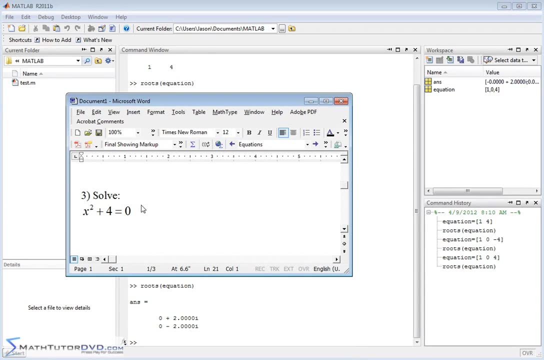 You always expect to get these conjugates in pairs like this, And just to make sure that this makes sense, if you move the 4 over here, it should be negative 4.. Take the square root. It would be plus or minus the square root of negative 4.. 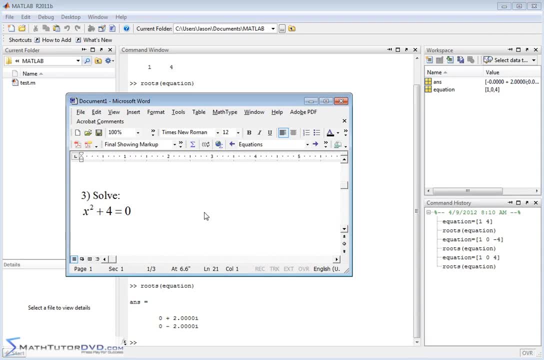 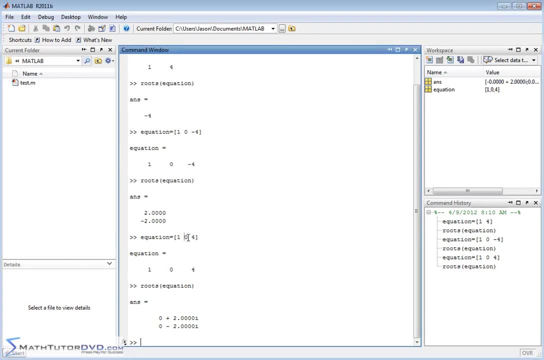 And so you're going to get a pair of imaginary answers there. So that's exactly what happens. The only thing you need to make sure of is when you're setting up the coefficients here you need to make sure and put a 0 anywhere where there is no variable present in your 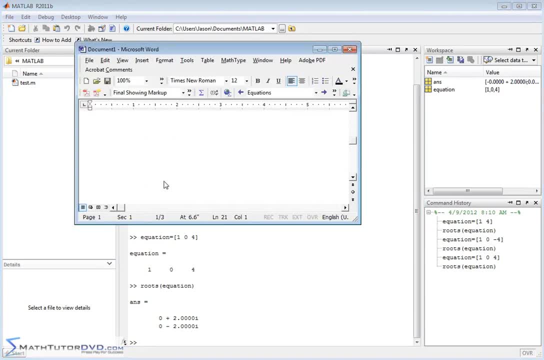 original equation. All right. So let's go down and solve an equation like this. So this is beta, Basically the same sort of deal. We have x squared minus 3x plus 9.. So let's go and set this up again, just for variety. 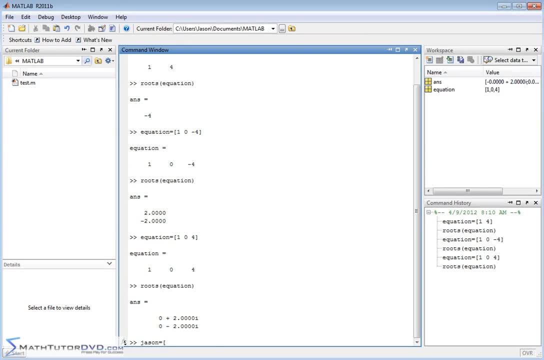 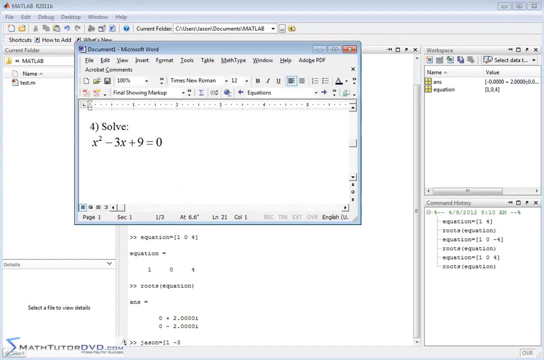 I'll name it JSON And I'll set up a single row matrix like this: x squared minus 3x, So it's 1x squared minus 3x And the last part of it was plus 9.. And that is the definition of what we're trying to solve here, because here we have x squared. 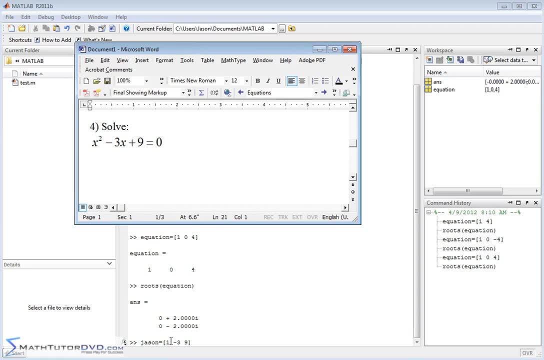 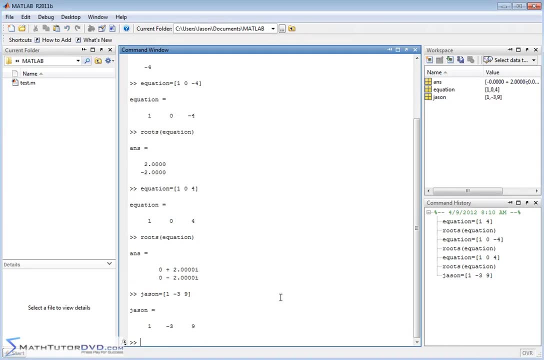 We have a term. in x We have a constant term, So there's no zeros. Everything is accounted for in our equation. Everything matches up coefficient-wise. So I will go ahead and define that little row matrix there And I'll do the roots command on what we just defined. 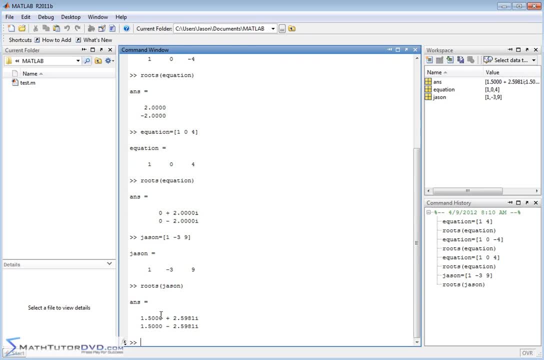 And again we get two answers which are complex conjugates of one another. The reason we get two answers is because this is a second-degree polynomial. We expect it to cross the x-axis twice In this case. it's a complex answer. 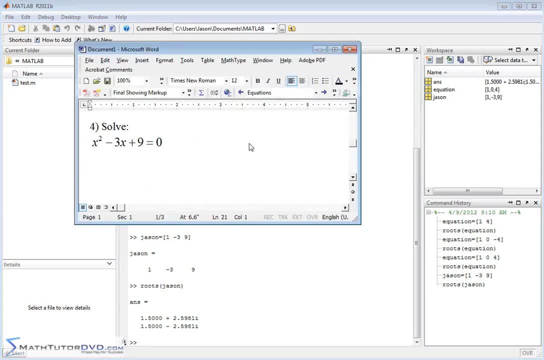 We expect to get two roots, All right. So that's basically how you do it, And you can put more complex answers. You can put more complicated things into MATLAB here. Here we have x to the fifth minus 3x to the fourth. 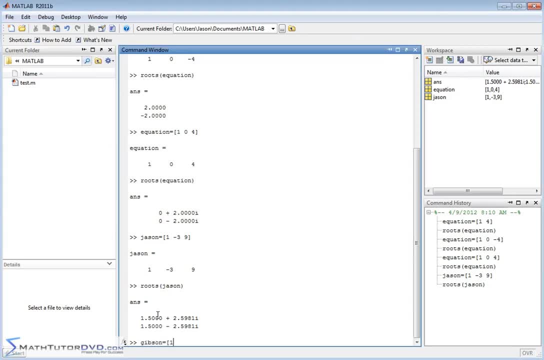 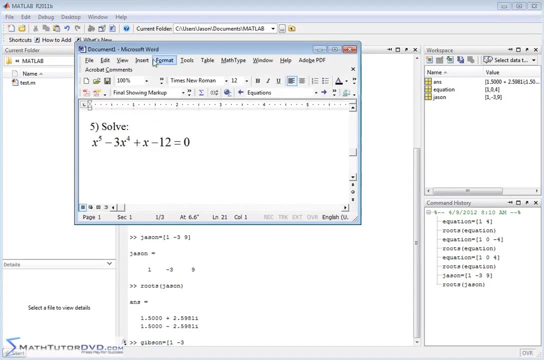 So I'll do my last name here. 1x to the fifth. Here we have negative 3x to the fourth, So I'll put a negative 3 there. Now there is no x to the third, So I'm going to have to put a 0 there. 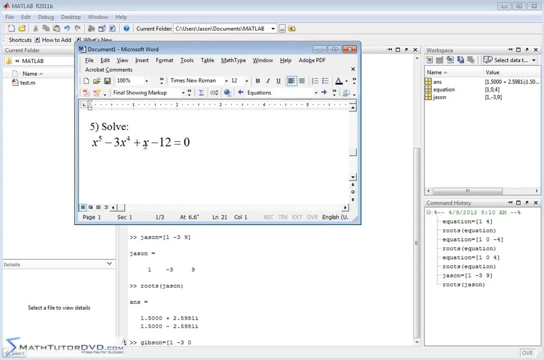 But then I'm going to have a 1. And there's no x squared also, So there's got to be another 0 in there, And then finally there's 1x, And then there's 1x squared, And then minus 12.. 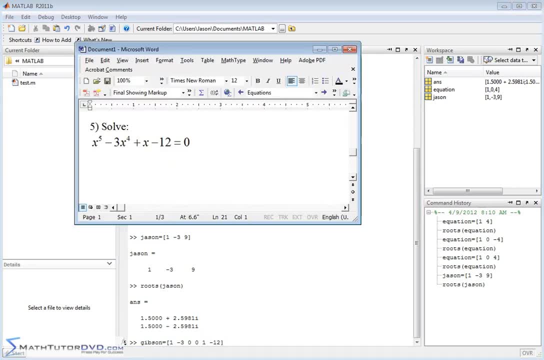 So 1 minus 12.. And make sure you understand how we arrive at this, because it's really the most important part of everything we're doing here: 1x squared minus 3x to the fourth plus 0x, cubed plus 0x. 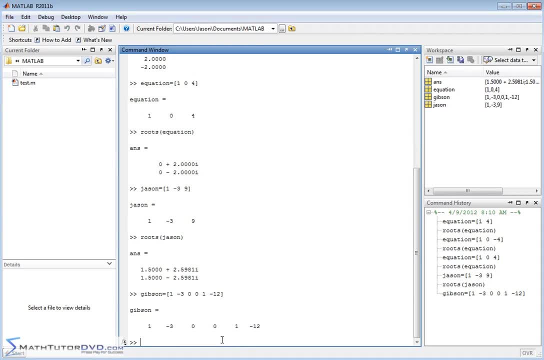 squared plus 1x minus 12.. We have to put 0s everywhere where we need that And then we'll do roots on this variable here And notice we get five answers. The reason we get five answers is because it's a fifth order. 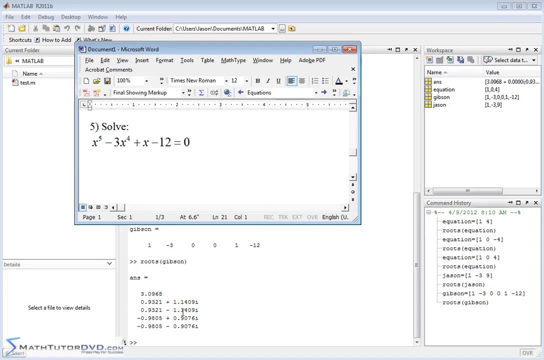 So, if you look at the table, let's note that we have three electrical moments. when something is- One of them- isід4- polynomial like this, One of them is real. The other four are complex conjugates occurring in pairs, which always is the way algebra works. 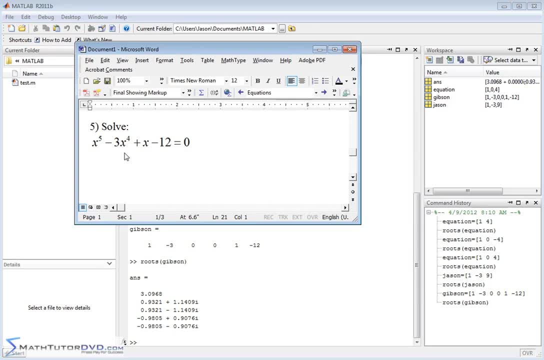 So so far we've been using the roots command. It's pretty powerful Most of the time. you're trying to solve a quick equation, a quick polynomial equation. This is the way you're going to do it. Now, notice that I've set all of these equations up equal to 0,. 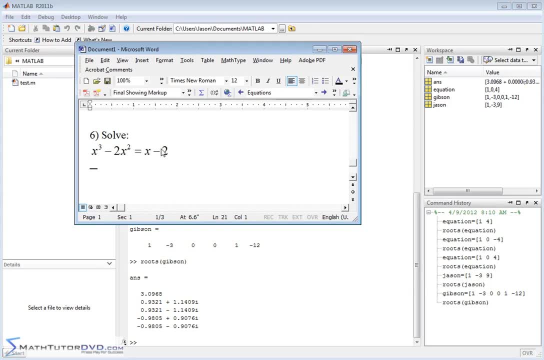 but just to kind of make sure you understand, So plain�� is equal to something on the right hand side and it's not equal to zero, then what you need to do is mentally sort of move one half of it over to the left hand side so that it. 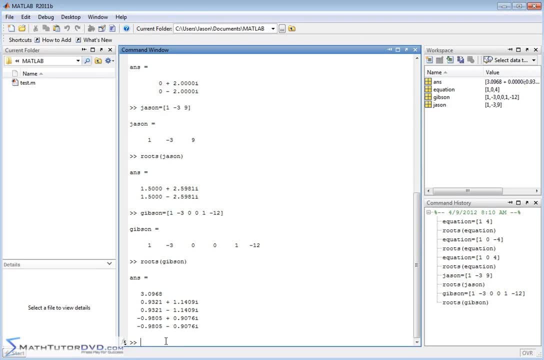 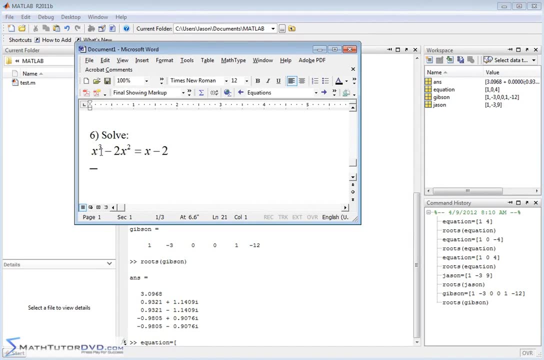 is equal to zero. So, for instance, if I wanted to do you know equation and set up a matrix, again set up the coefficient matrix, then on the left hand side it's going to be 1x cubed minus 2x squared. 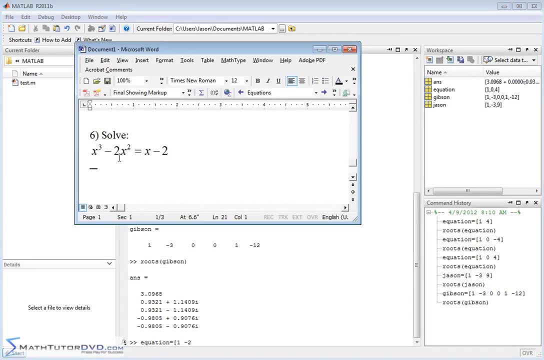 So it's 1x cubed minus 2x, squared like this. and then when we move the x over here it's going to be negative 1x, so I'll have a negative 1x, And then when I move the negative 2 over, that's going to become a positive 2, so that's. 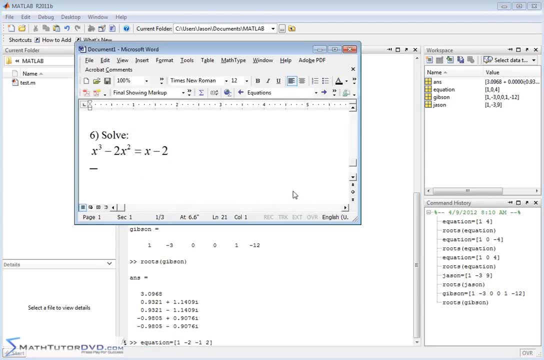 going to be a positive 2.. And this is how I set up my coefficient matrix for this problem. I'm just trying to let you know that it doesn't have to be equal to zero. you just take what's on one side, you move. 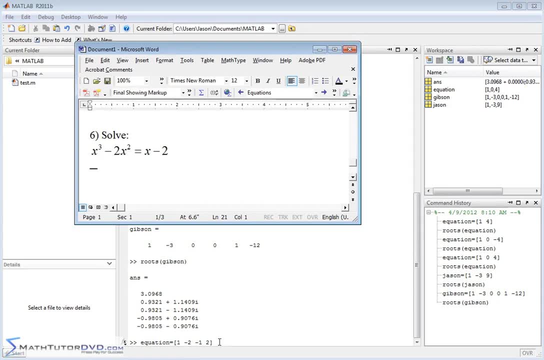 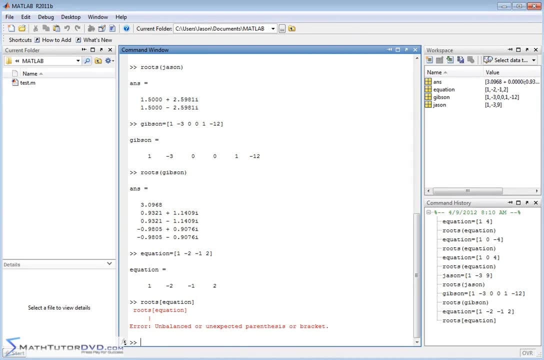 it over and then you have the coefficient set up appropriately and then you just go ahead and solve the problem. So roots of equation and in this particular case, in this particular case, it's a good example of of what not to do. you notice, I tried to pass the equation variable inside of brackets. 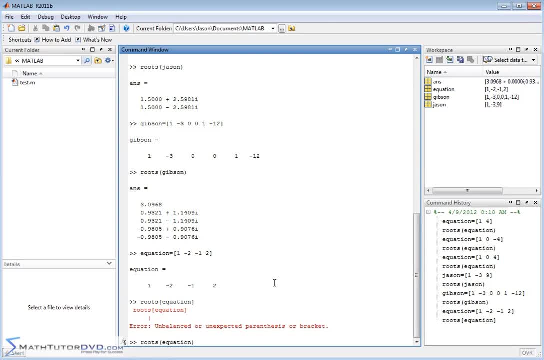 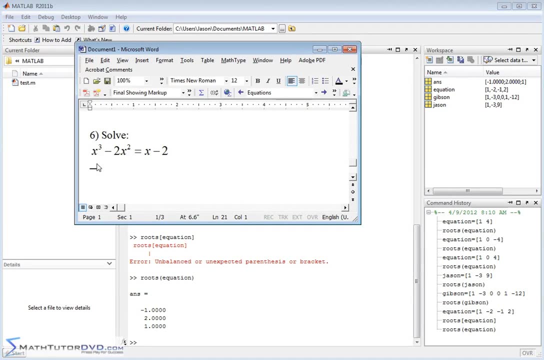 So if you ever do something like that, don't get too worried about it, just do it the proper way, inside of parentheses, and then, in this case, we'll get three answers, and they're real numbers. in this case, The reason we get three answers is because we have a third degree or a third order polynomial. 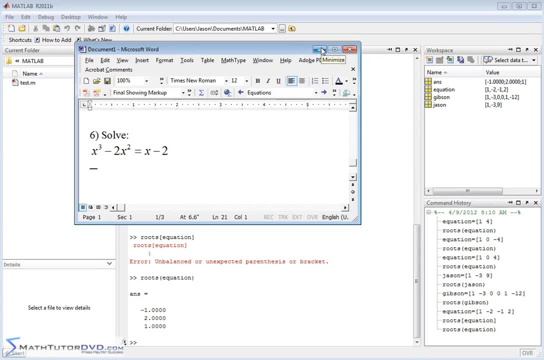 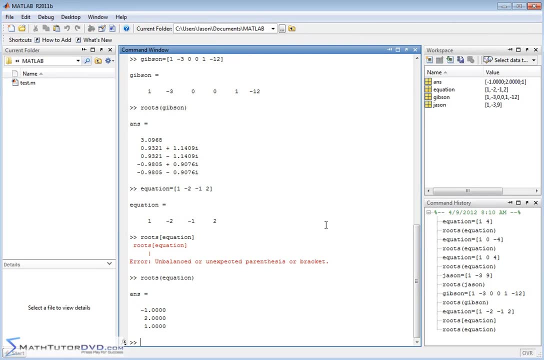 like this. So this is, you know, a really great way to solve quick, simple algebraic equations. A lot of times you're you're doing a project and and and so inside of a program or something, you need to solve an equation. 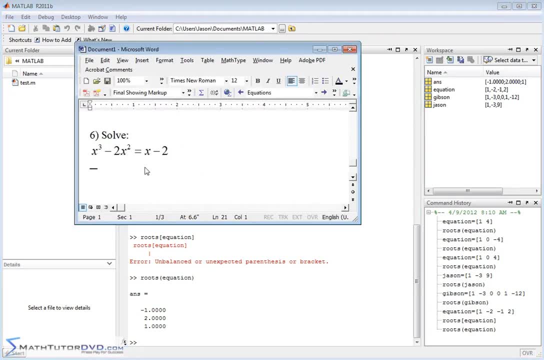 Lots and lots and lots of equations are linear like this. you know that you need to end up solving quickly. or maybe your coefficients change as you're going through your problem. you know, and your, your program is adjusting the coefficients and you need to quickly solve. 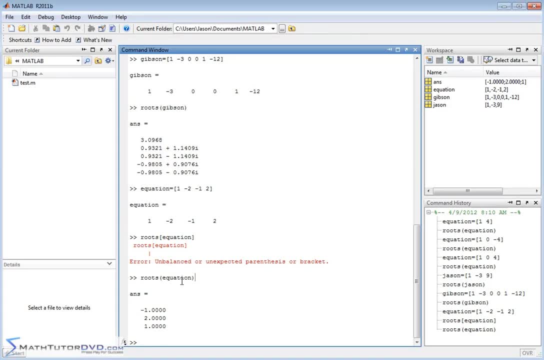 them. The roots command is a very quick, fast way to do that. The only thing is you have to define the equation. you don't type it out: 3x squared plus 2x, you have to give it the coefficients. MATLAB is basically a matrix sort of animal.